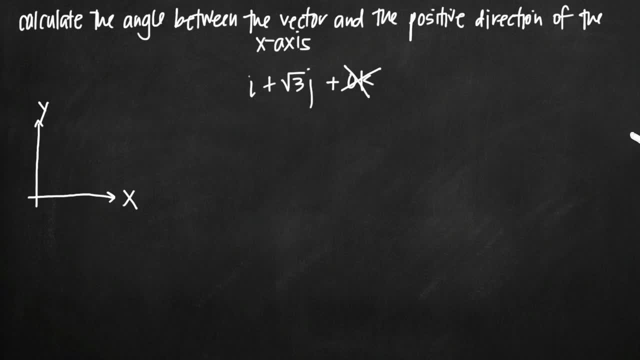 of 3j can be represented by this vector here. First we need to recognize that we have a coefficient on our i component here of 1.. Right, we have 1i plus square root of 3j. Remember i corresponds to the x component. so what we can do is go out along the x-axis. 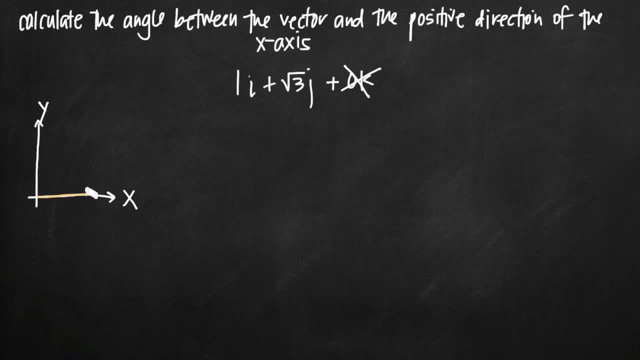 a distance of 1.. So let's pretend here that this is a distance of 1 along the x-axis. Then our j component more or less corresponds with y, our y variable. So we want to go up a distance of square root of 3.. 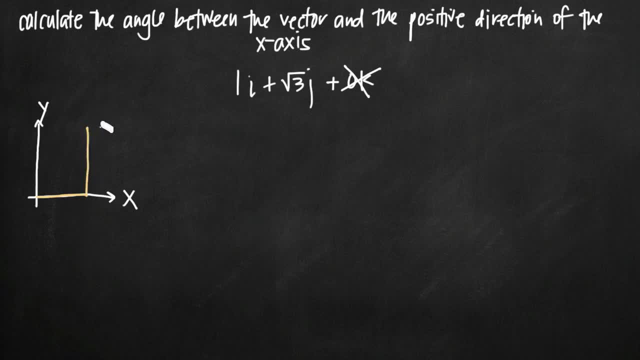 So let's pretend that this is a distance that represents square root of 3.. Well, if we just connect our initial point at the origin and our final terminal point here, then that's going to represent the vector i plus square root 3j. 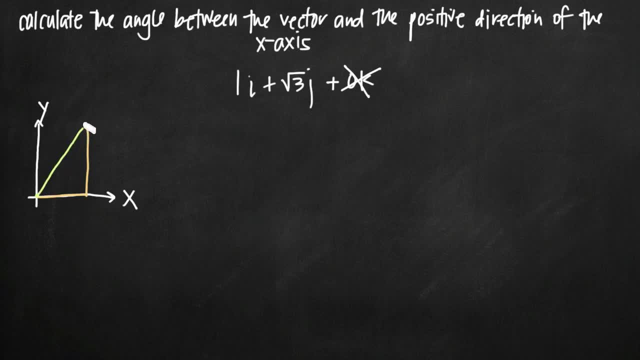 We'll start here, at our initial point, we'll go to our terminal point here, and this is the vector i plus square root of 3 times j. Now a couple things that we know about the triangle here that we've created. First of, 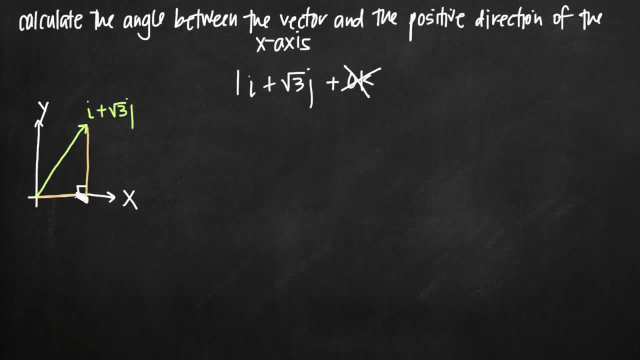 all, we have a right triangle here, with this angle being 90 degrees. We also know that we're looking for the angle between the vector and the positive direction of the x-axis. That's going to be this angle here And we'll go ahead and represent that here. So we're going to go ahead and represent that. 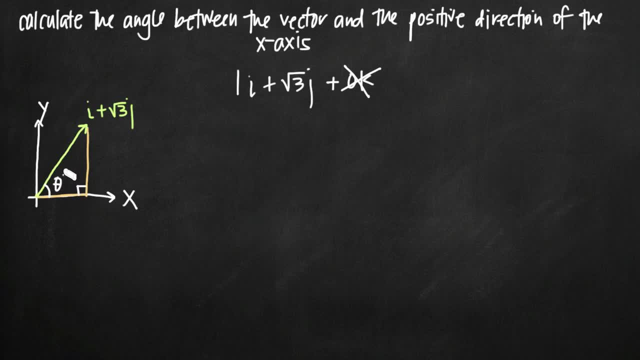 angle with the variable theta. This is the angle here that we want to find. We know that this side of our triangle is a length of 1, and that this side of our triangle is a length of square root 3.. Given two sides, 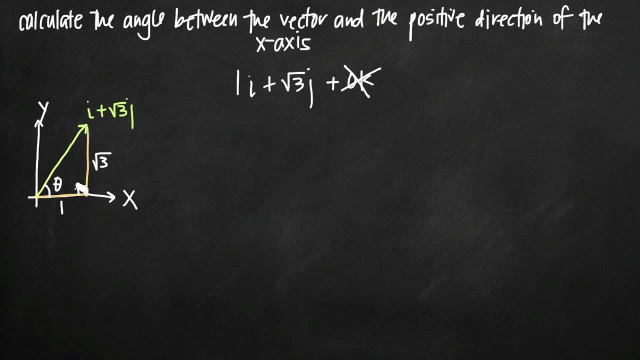 of our triangle. we can find the value of this angle Because, in comparison to the angle, we have the length of the opposite side right- this is the opposite side- and we have the length of the adjacent side. This is the adjacent side. 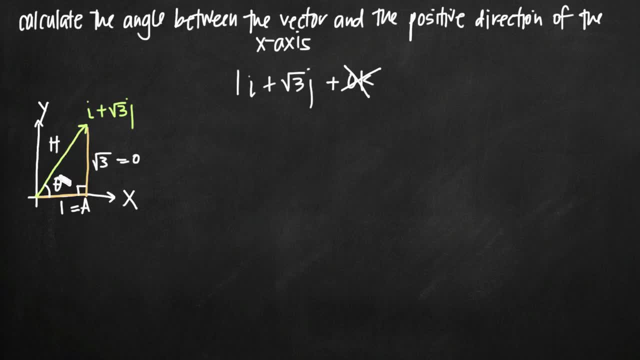 Right, And which function of the angle theta is proportional to the length of theta. Well, this is our prime and we have the length of the opposite side. We're going to find that ourа is equal to the length of the adjacent side. Remember that the tangent of the angle 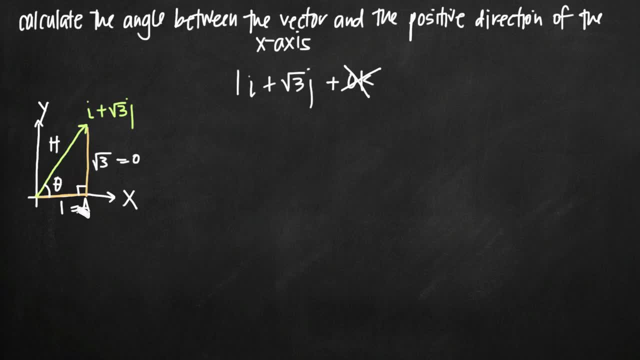 theta is equal to the length of the opposite side divided by the length of the adjacent side. so what we can say is that tangent of theta is equal to the length of the opposite side, square root of 3, divided by the length of the adjacent side, which is 1.. 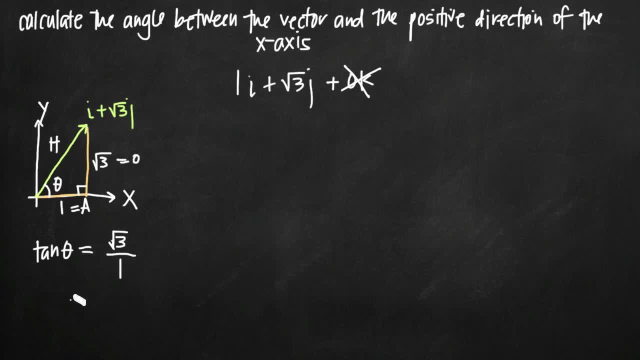 All we need to do at this point is figure out how to store the angle actually, and this is what we're going to find- For example, we're going to use the angle theta as a sum of. So the first thing we want to do is just simplify and say that tangent of theta is equal to. 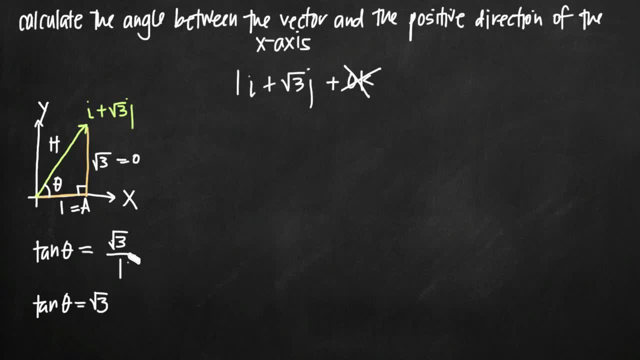 square root of 3.. No need to write square root of 3 divided by 1. That's redundant. So tangent of theta equals square root of 3.. Remember that tangent is equal to sine divided by cosine, So we can replace tangent of theta with sine of theta divided by cosine of theta equal. 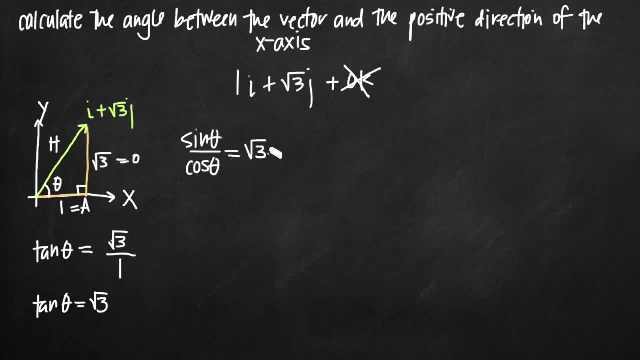 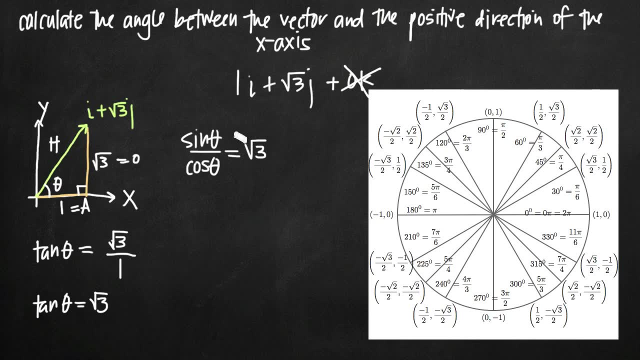 to square root of 3.. Now here's where our unit circle gets involved. We need to find a value for theta such that when we take sine of theta, the value of sine of theta, and we divide it by the value of cosine of theta, our result is square root. 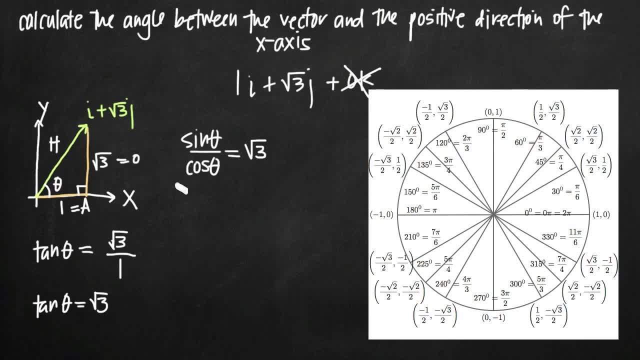 of 3. Because our vector starts at the origin and moves through the first quadrant here of our two-dimensional coordinate system. we want to look at values along the unit circle in order to find the value of sine of theta. So we want to find the value of sine of theta in our first quadrant. 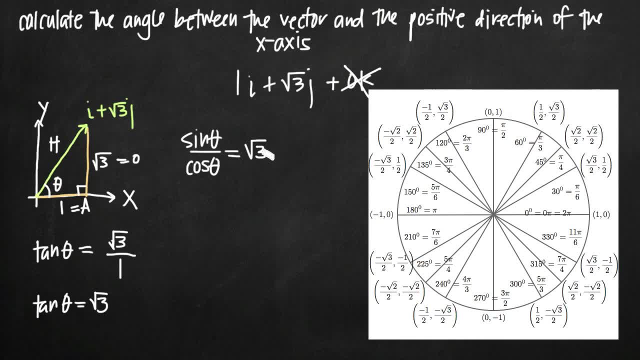 Well, which of these three coordinate points here in our first quadrant are likely to give us a result of square root of 3 when we divide the y value of the coordinate by the x value? Remember that the y value is associated with sine. The x value is associated with cosine. 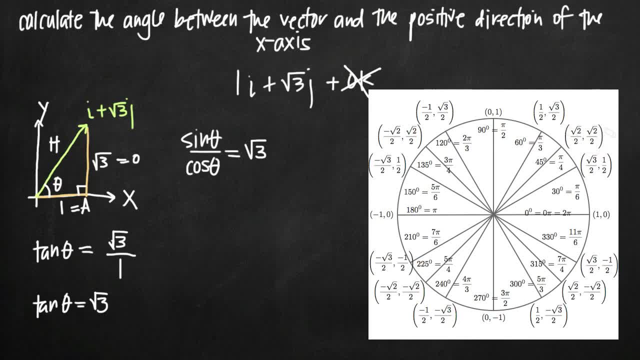 Well, probably not square root of 2 over 2 divided by square root of 2 over 2.. That would just give us 1.. There's no square root of 3 value involved there. We're not going to use this coordinate point here. 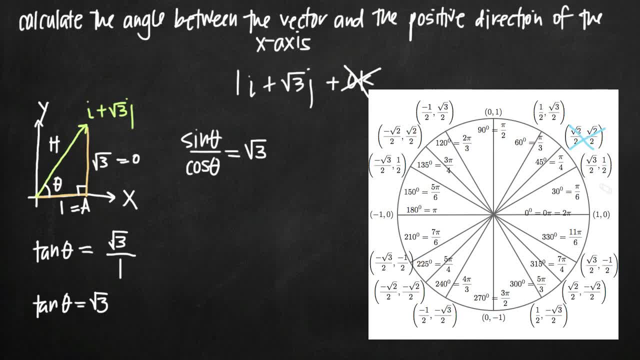 These two are both candidates though. So if we took, for example, theta, equals pi over 6, this first angle right here, and we took the value for sine, the y coordinate, so 1 half, and we said 1 half divided by the. 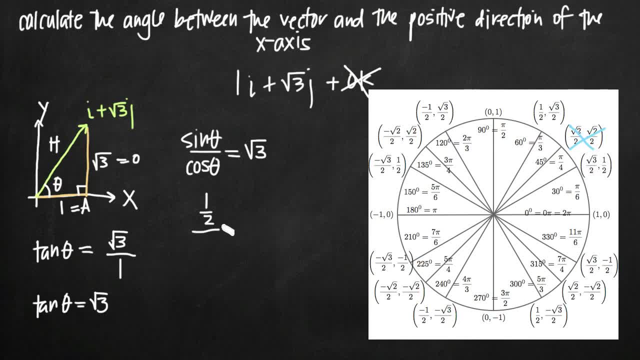 value for cosine, the x value, which is square root, of 3 over 2, divided by root- 3 over 2, what that would give us, instead of dividing by this fraction, we'd say 1 half multiplied by the reciprocal. 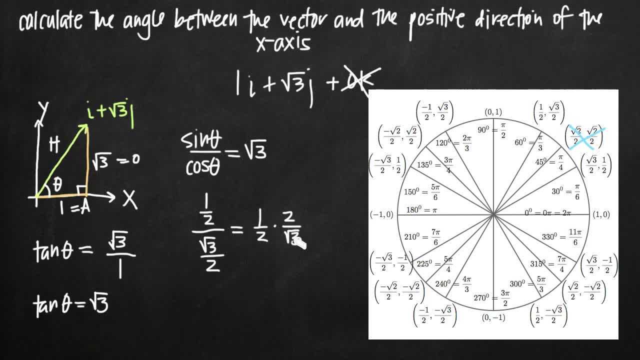 We'd flip it upside down and do 2 over square root 3.. When we get that result, obviously we get the 2s to cancel and we get 1 over square root 3.. Well, that's not quite our square root 3 value. 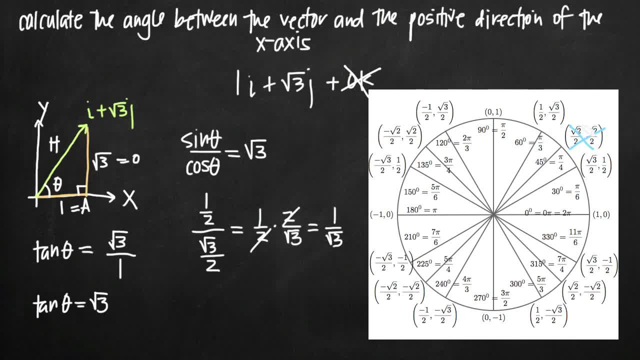 What if we do this other one, pi over 3?? Well, in that case we take the sine value, square root of 3 over 2, that's the y value, so square root of 3 over 2, and we divide that by the cosine value, which is the x value. 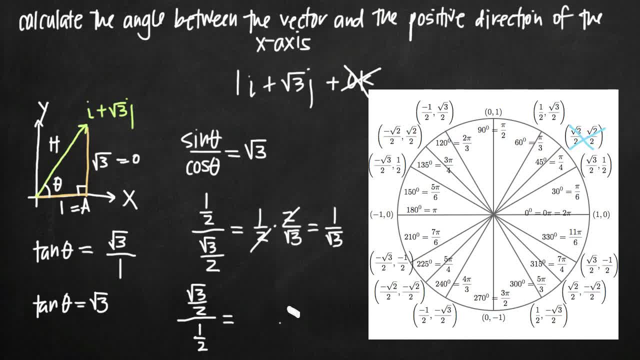 1 half, so 1 half here. When we simplify, instead of dividing by the fraction, we'll multiply by its reciprocal. so we flip the denominator upside down. Instead of 1 half, we do 2 over 1, and we get our 2s to cancel, and we're just left. 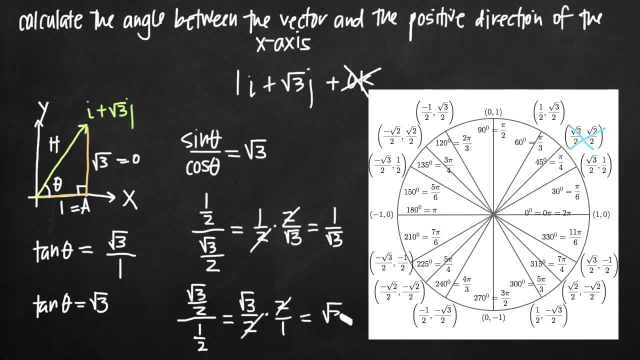 with square root of 3 over 1, or root 3.. Perfect, That's what we had originally here: sine of theta over cosine of theta with square root of 3.. So we know now that we've found our matching value here: root 3, that theta over cosine. 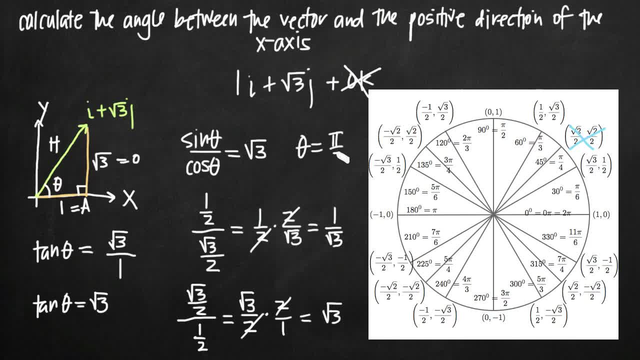 of theta is going to be equal to pi over 3, which is the same as 60 degrees. so we can say 60 degrees here. Now you might realize one thing you might realize is that the value on the unit circle 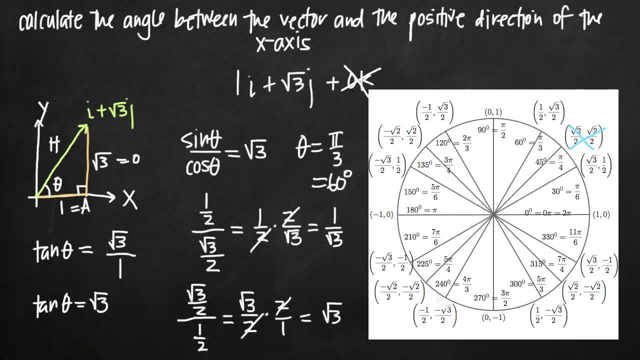 down here at the angle, 4 pi over 3, where our coordinate is negative 1, half negative root 3 over 2, that if we used that value for theta that we would get a value of positive root 3.. So you might think that 4 pi over 3 was also an acceptable value of theta. 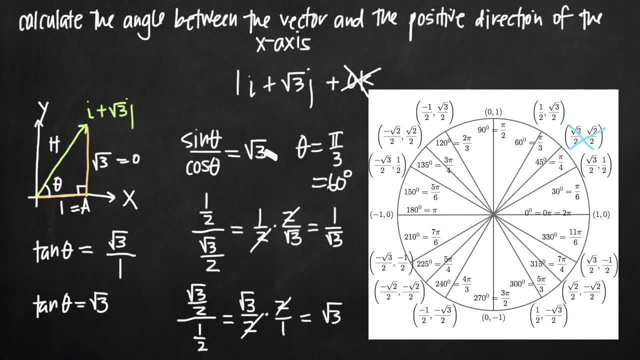 However, it really isn't an acceptable value of theta because, even though it gives us root 3, here our vector is in the first quadrant. We have a positive x value right. This is positive 1, which tells us to move one unit in the positive direction along the